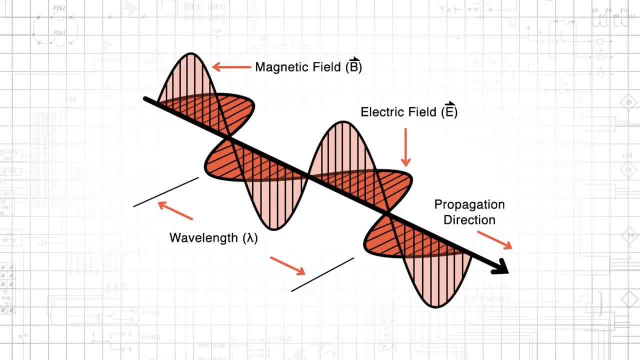 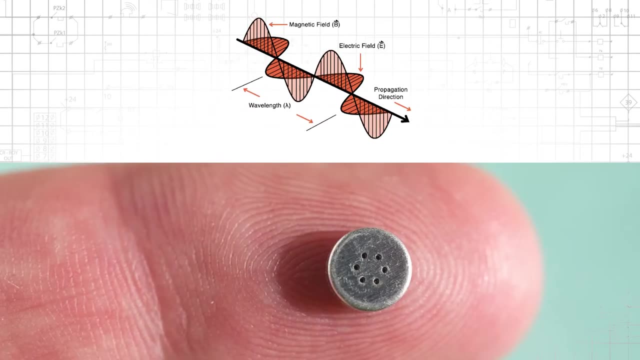 mechanical components, monitoring physical processes generating or receiving electromagnetic signals, and analyzing environmental variations. Sinusoidal relationships are present in the world that surrounds an electronic device and consequently, many electronic devices incorporate sinusoidal signals. Sinusoidal signals figure prominently in the work of electrical engineers. 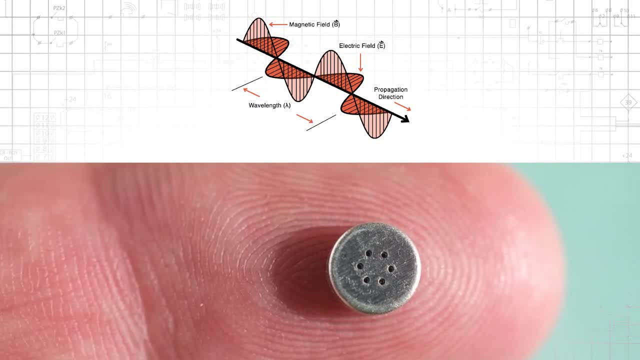 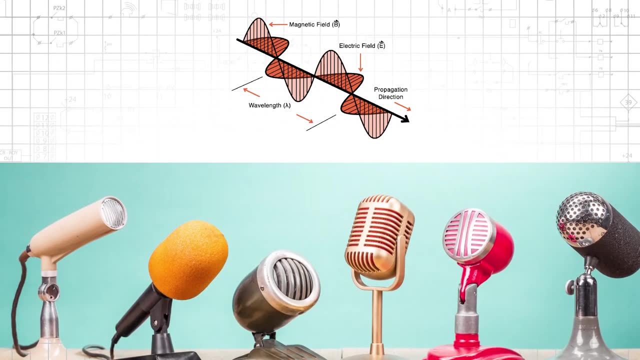 who design audio systems. Microphones generate sinusoidal voltage signals that correspond to variations in air pressure. These are delivered to amplifiers, which produce sinusoidal signals that can be analyzed, modified or stored for later use. Power amplifiers convert sinusoidal 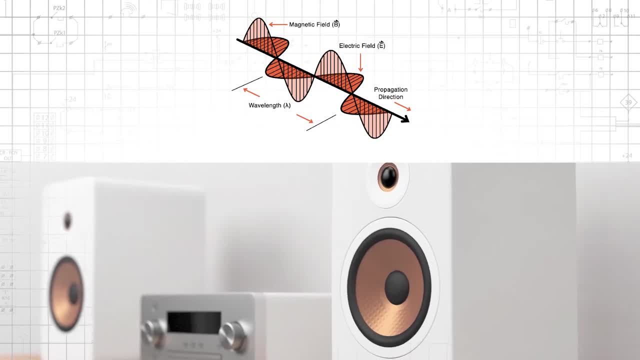 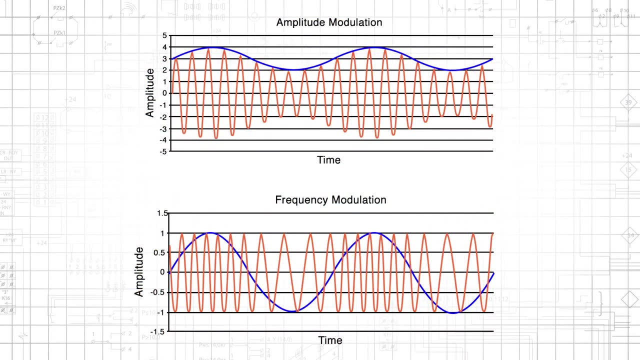 voltages into signals that can drive a speaker, and speakers convert sinusoidal signals back into air pressure variations. Radio systems make wireless communication possible by generating sinusoidal signals that produce electromagnetic radiation that can travel long distances and pass through solid objects. Special modulation techniques are used to modify sinusoidal signals. 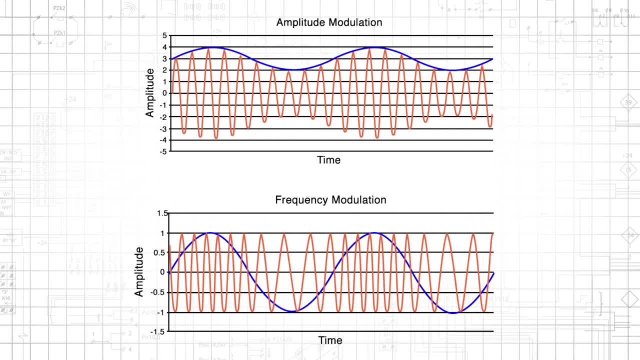 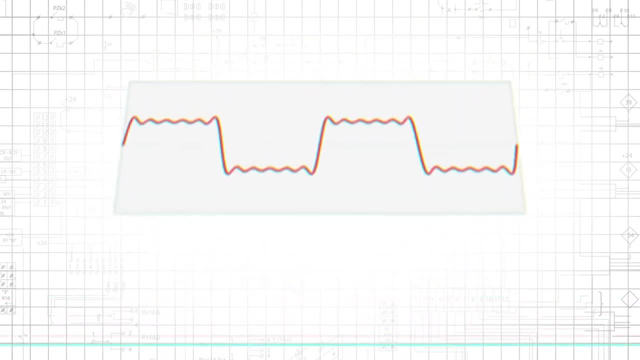 such that they can carry information from a transmitter to a receiver. RF engineers use amplitude, frequency and phase as modulation variables. Changes in the signal range can be transferred as electromagnetic radiation, recovered by an electronic receiver and interpreted as an information-bearing signal. Some very interesting applications of sinusoids: 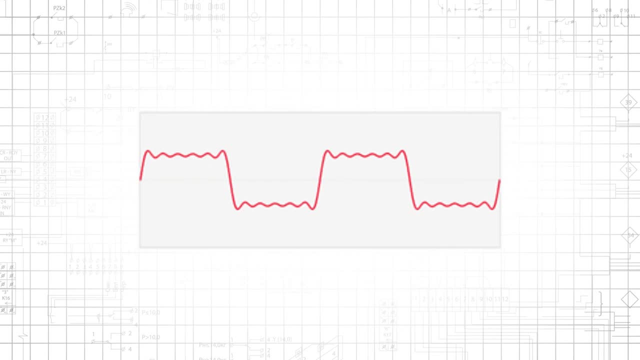 take place in circuits that don't have sinusoidal signals, or at least the signals do not appear to be sinusoidal. It turns out that electrical signals can be analyzed as though they are produced through the addition of multiple sine waves with different frequencies and amplitudes. This concept is based on the Fourier transform, which is a mathematical process. 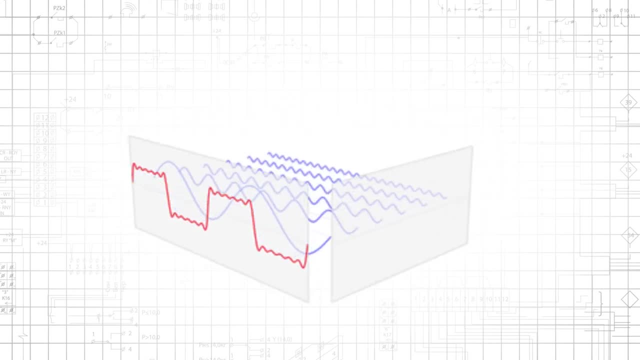 that converts sinusoidal signals to electromagnetic radiation. For example, if you have a sinusoidal signal, you can convert a normal signal into a series of sinusoids that represent the signal's frequency content. When we analyze a signal as an amplitude that varies with